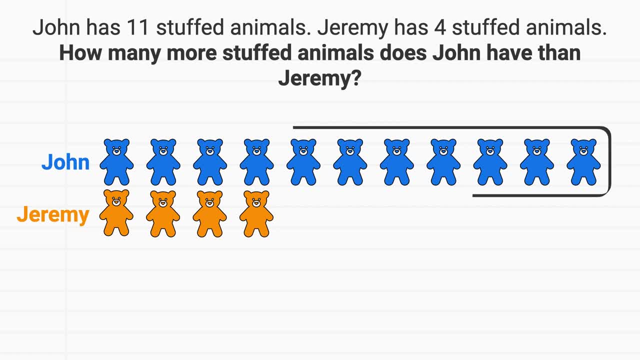 how many more John has. That's this quantity. here It's the stuffed animals that John has, but Jeremy doesn't. Well, we could count that John has one more, two more, three more, four more, five more, six more, seven more. John has seven more stuffed animals than Jeremy. 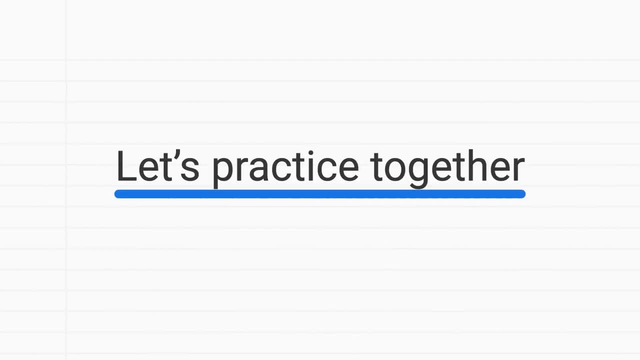 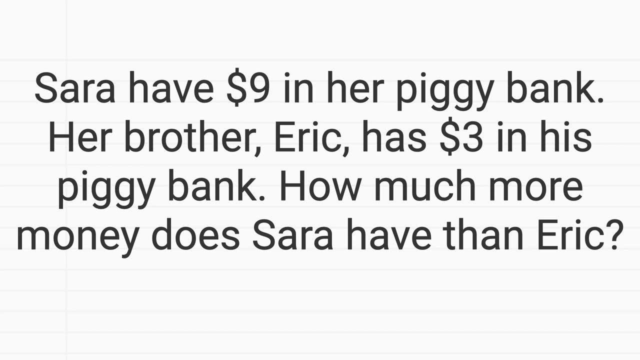 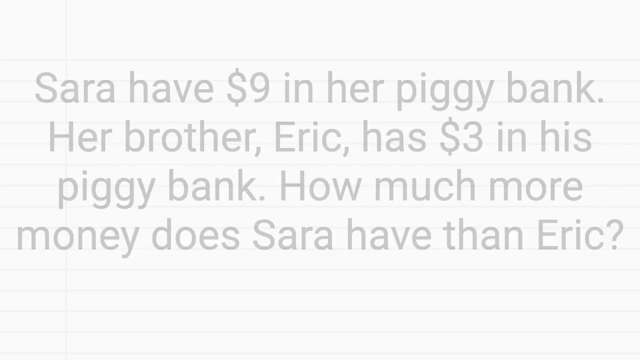 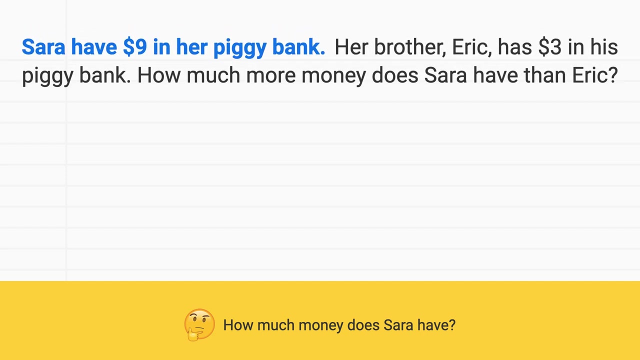 Now let's practice one of these together. Sarah has $9 in her piggy bank. Her brother, Eric, has $3 in his piggy bank. How much more money does Sarah have than Eric? Well, if we think about this problem, how much money does it say Sarah has? It tells us that Sarah has $9 in her piggy. 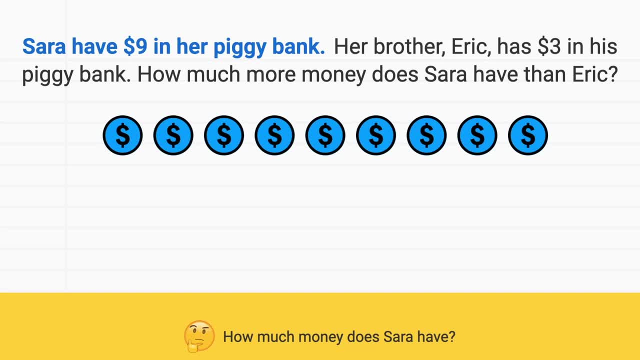 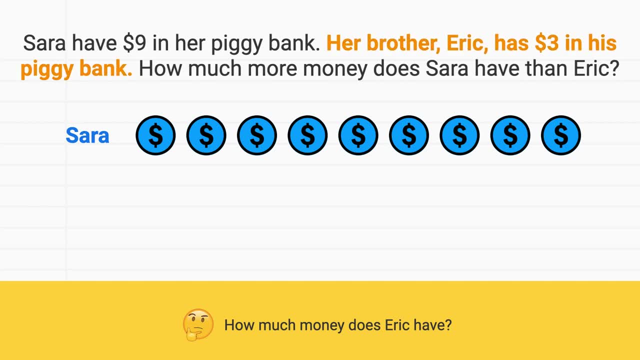 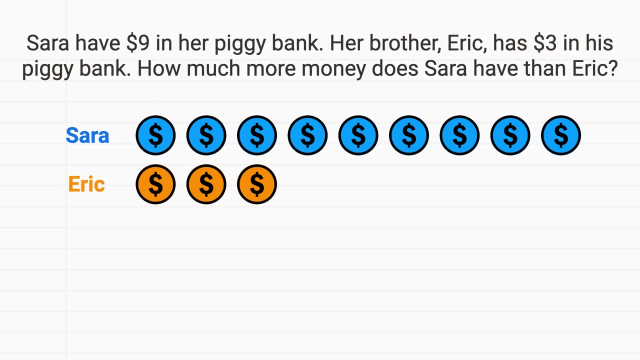 bank We could draw out those $9.. These are seven dollars. Now let's practice one of these together. Sarah's Then. how much money does Eric have? The problem tells us her brother Eric has $3 in his piggy bank. Here are Eric's $3, and we'll label them as his. Now we need to solve how much more. 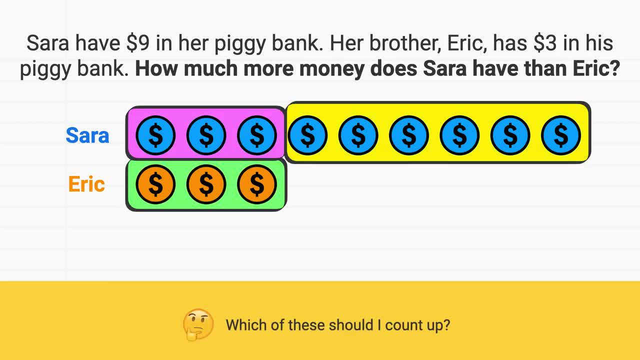 money does Sarah have than Eric? Well, which of these quantities could I count to find my answer? We will count up this quantity. This is the money that Sarah has, but Eric has $9 in his piggy bank. How much more money does Sarah have than Eric? 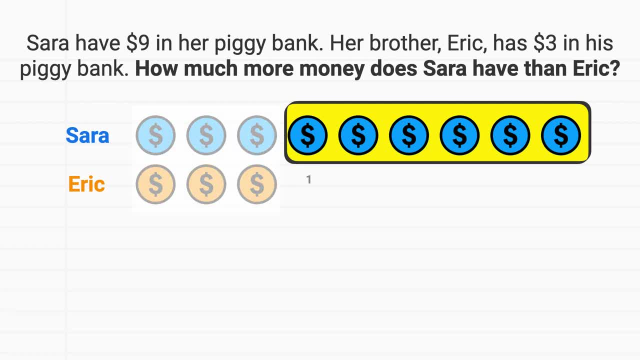 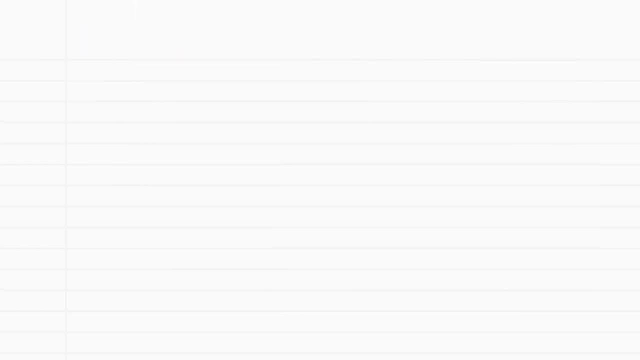 Eric does not. Well, we could count. Sarah has one more dollar, two more dollars, three more dollars, four more dollars, five more dollars, six more dollars. We would say Sarah has six more dollars than Eric. Now it's time for you to practice one of these on your own. What is the? 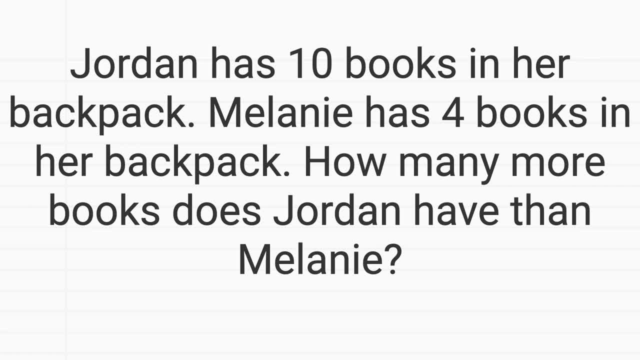 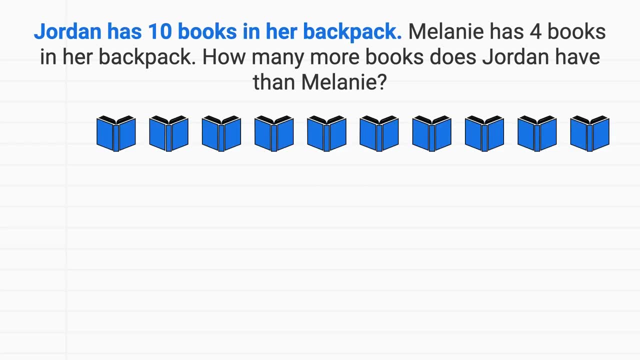 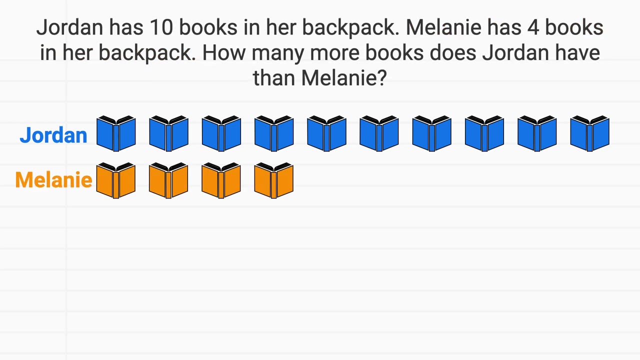 answer to this problem. Jordan has 10 books in her backpack. Melanie has four books in her backpack. How many more books does Jordan have than Melanie? Well, in this problem we can start with Jordan and her 10 books. Here are Jordan's 10 books. Then we'll draw out Melanie's four books Now to find. 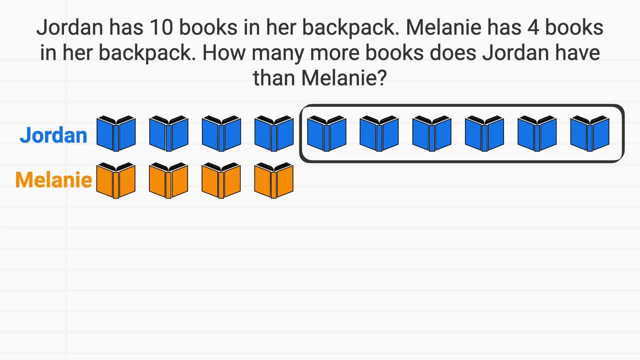 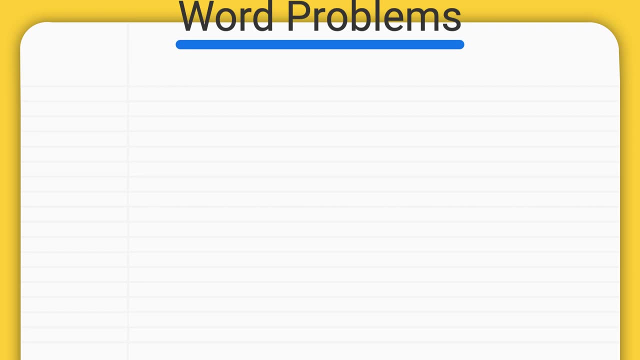 how many more books Jordan has. we'll count this quantity here. We can see that it's one more book, two more books, three more books, four more books, five more books, six more books. Jordan has six more books than Melanie Today. you learned how to solve word problems involving comparisons.